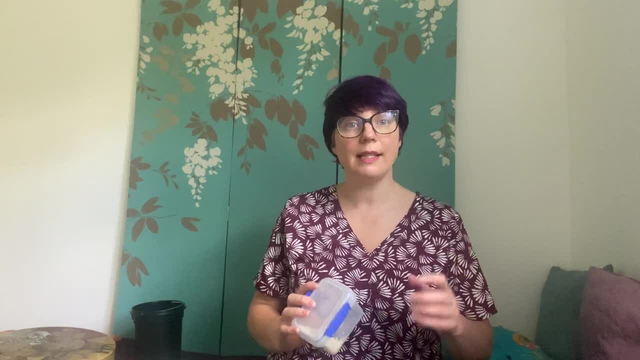 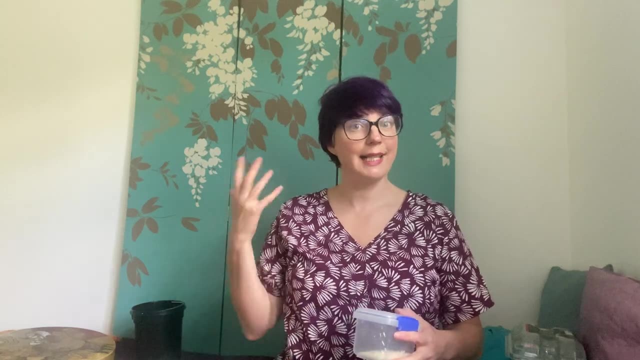 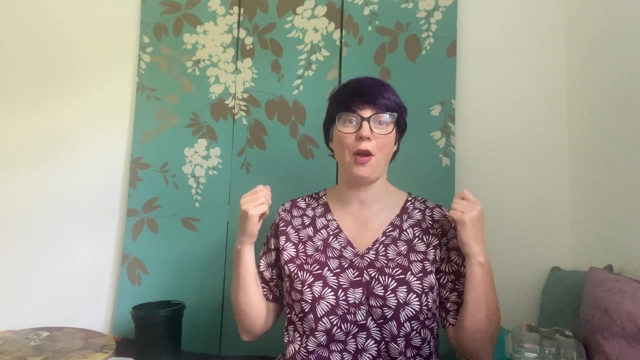 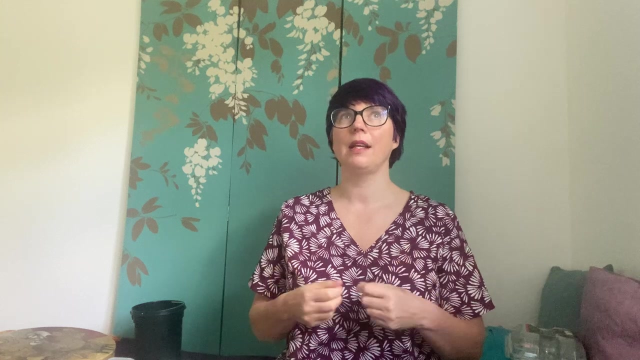 rice in it. It's a lighter sound, So have a play around with what sounds you like to hear. You don't want anything too jingly jangly on the ears because it could get- it can get loud. So we're trying to find sounds that are quite soft and non jarring. Otherwise, rather than being a fun, 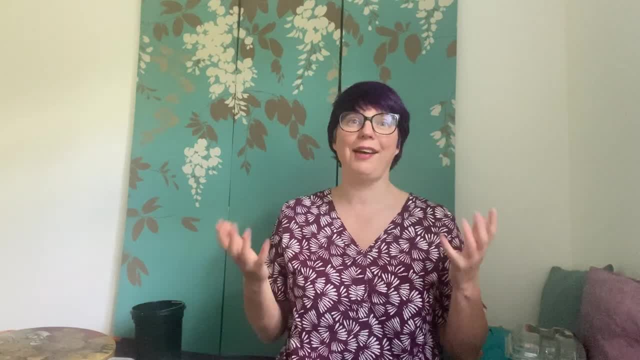 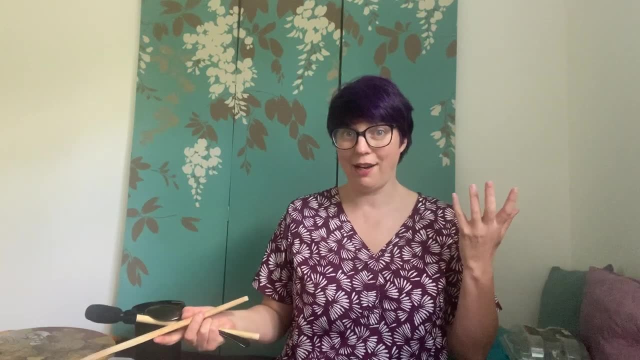 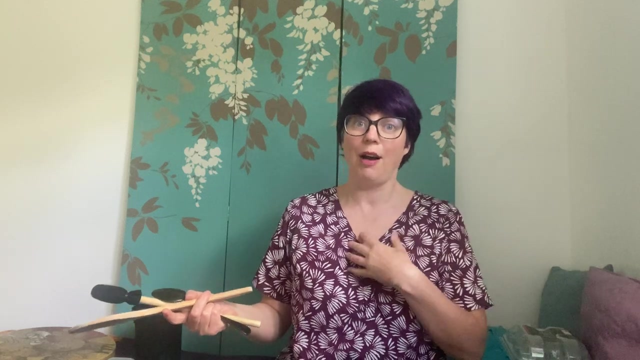 session. it will be like what's the word Overwhelming session- If you find you do have really sensitive hearing and you know the children you're with really want to sort of make lots of noise and actually it's too much for you. I personally have tinnitus, so I understand. 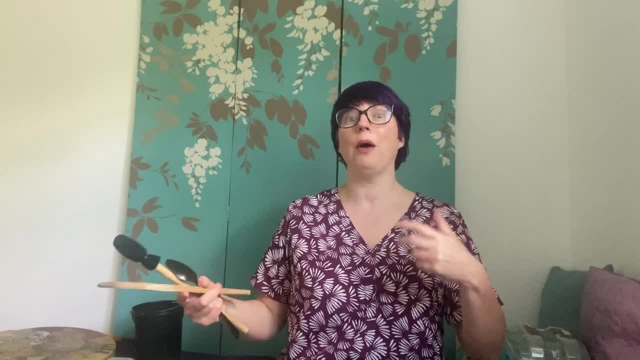 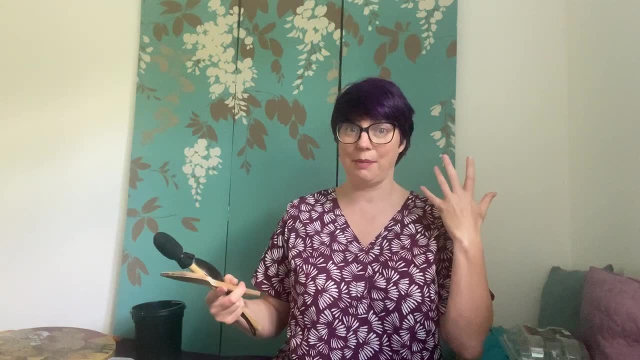 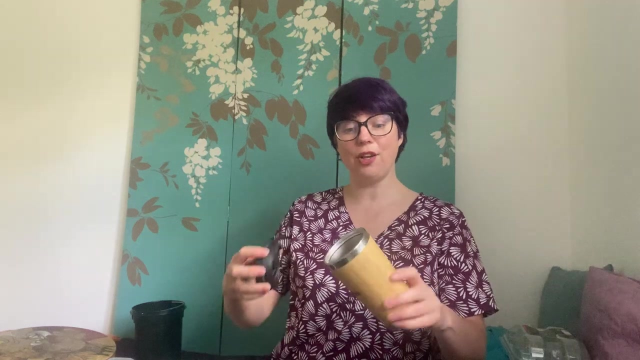 I do put tissue in my ears or earplugs. in That way everyone gets all the benefits of the loudness and the sound. So that way my ears and my nervous system don't get too jangled. So another container you might like to use: I've got a coffee cup And you can put some pasta. 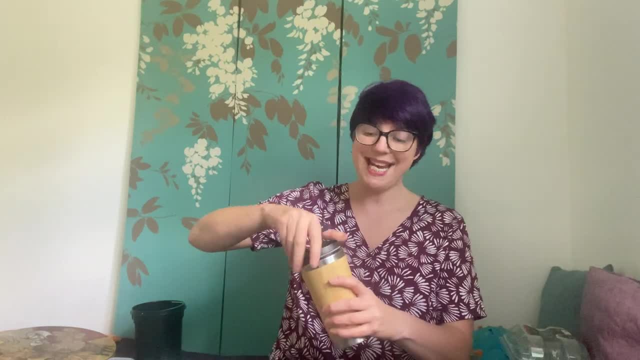 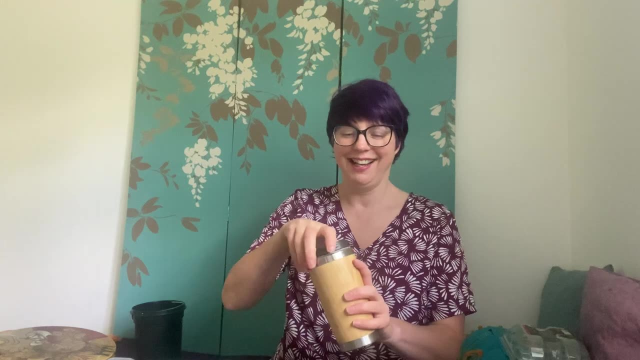 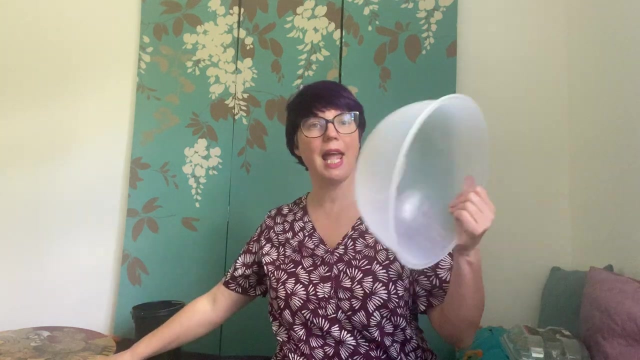 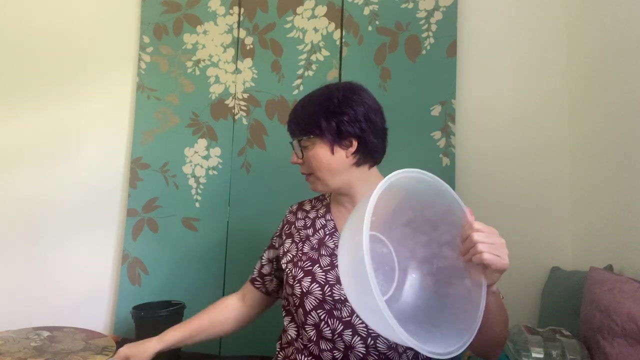 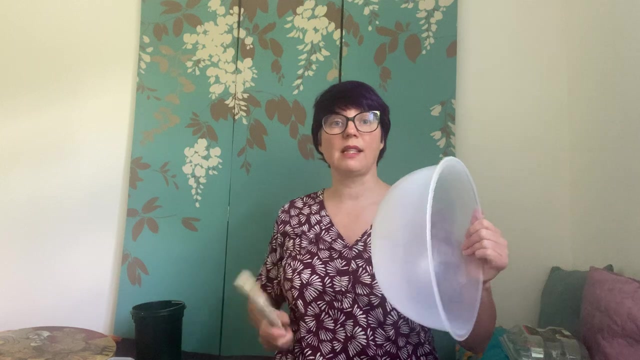 some stones, some beans. Give that a quick shake. Yeah, that's a little bit tinny for me. Personal preference: Whatever works for you, Awesome. Yeah, We have a plastic mixing bowl banging with a spoon, wooden spoon, a stick. So again, 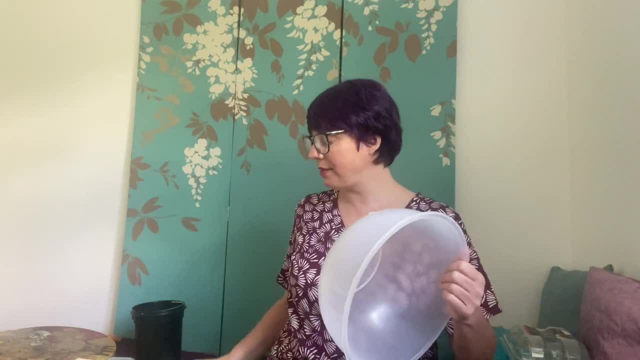 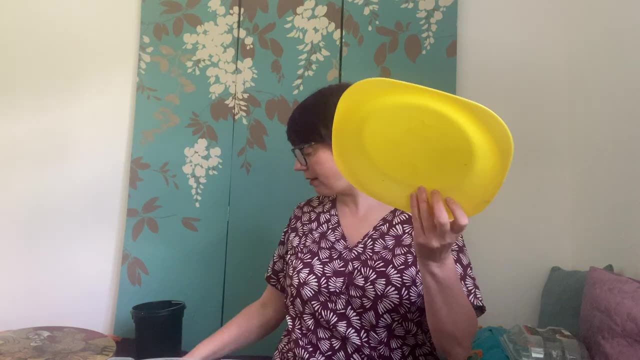 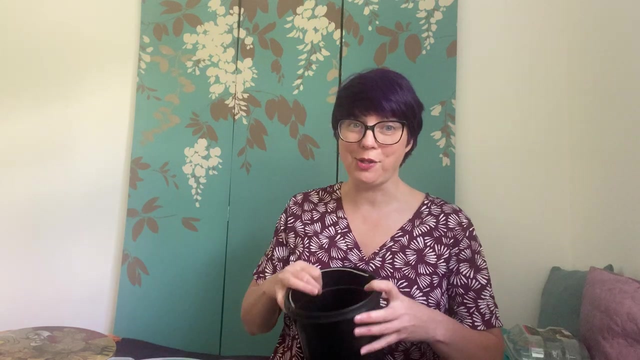 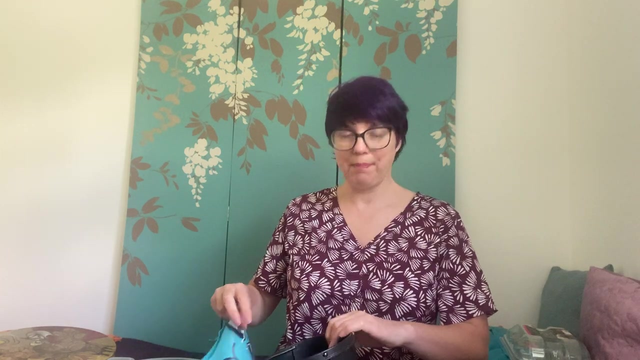 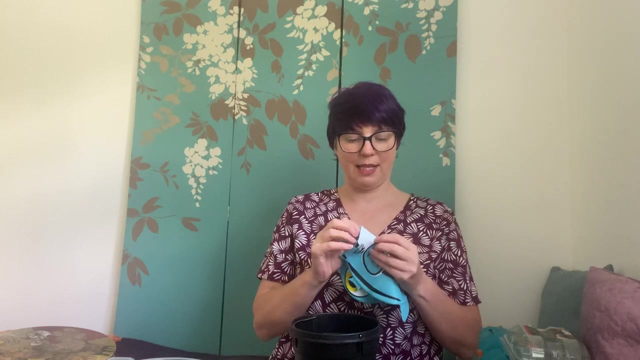 different sort of implements make different sounds, So it's quite fun to play around with that. Got a plastic plate. I did pick up a good little tip from one of the videos on YouTube, which is a little bin that I pinched from the bathroom and a swimming cap. I'm putting this over the top of the bin.